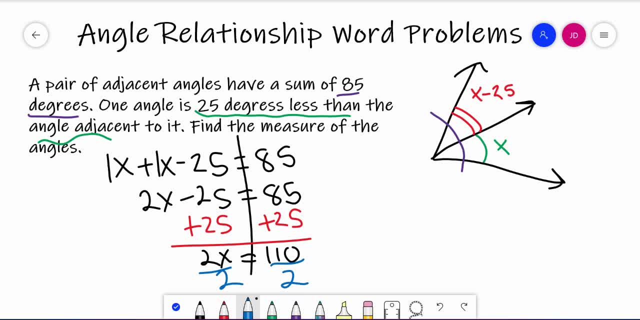 And now this: get's any greater or equal to zero And you're going to get: your x is 55. So that is the measure of this angle right here: 55 degrees. And to find the measure of this angle right here you have to do 55 minus 25.. 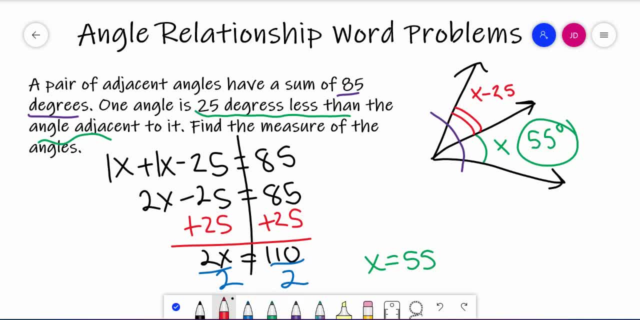 So 55 minus 25 is 30 degrees. And then when I add those two numbers together, you're negative. So you're going to have your x minus two times plusχ and overnight degrees. kind of plug into this all this angle right here. 55 is, And then when you'll find your x minus 20 degrees, in�� all these letter per cent, this is equal to 55 degrees and you'll have all your diseases enabled Alright. so 55 proper Rabbits with intelligence. So the measure of this angle 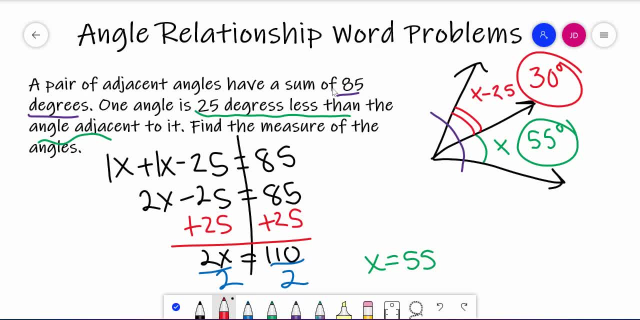 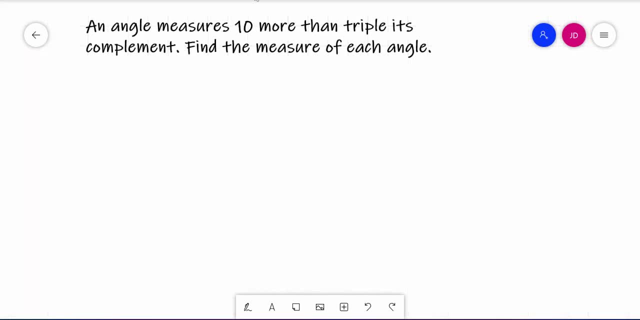 you get- you guessed it- 85 degrees. so that's a good way to double check your answer at the end. all right, let's look at another one. all right, so an angle measures 10 more than triple its complement. find the measure of each angle okay. complementary angles are two angles that add up to 90 degrees all. 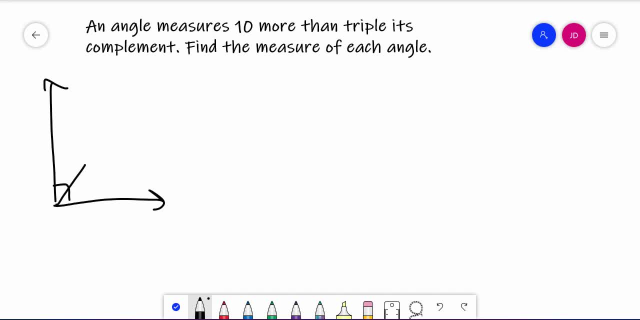 right. so I have two angles. one is this: one is ten more than triple its complement, ten more than triple its complement, the the. this one right here, we don't know- is X. so I create my equation: X plus 3x plus 10 equals 90, line down the equal sign, combined like terms. yet 4x plus 10 is 90. 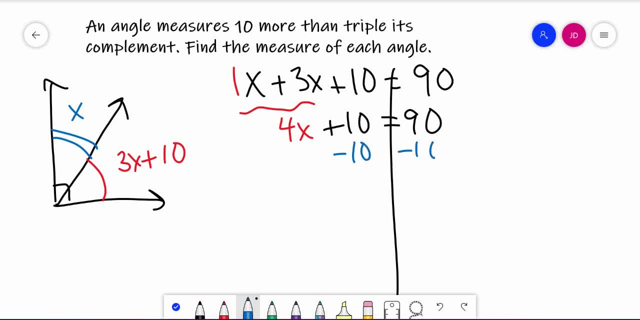 dealt. so it's negative時候 10 required. negative will the remembers minus 10 from both sides. and then we get 4x is 80. divide both sides by 4, which your X 20您, that's 20. that means this one is 3 times 20, which is 60 plus 10. 3 times 20 plus 10. 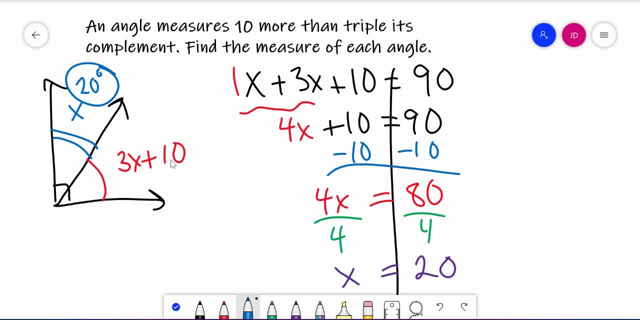 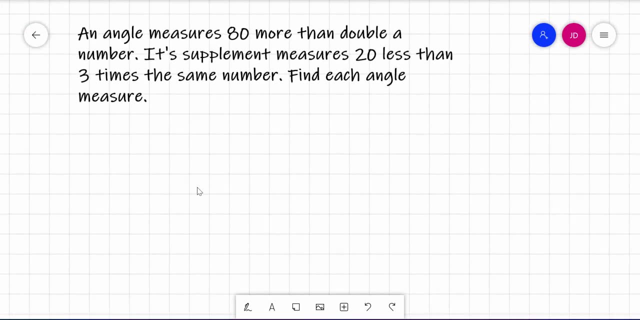 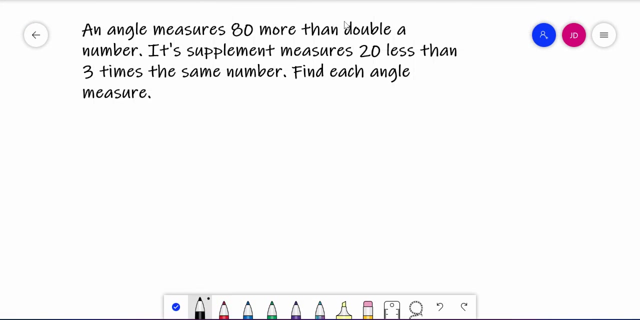 which is 70 degrees. so those are my two angles: 20 degrees and 70 degrees. alright, let's look at one more. okay, an angle measures 80 more than double a number. it's supplement, so supplementary angles measures 20 less than three times the same number. find each angle. 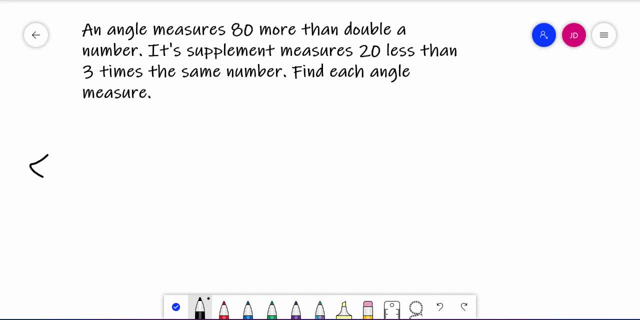 measure. alright, so I have supplementary angles. that is another way. supplementary is a straight line there form a linear pair. so I'm just gonna guese to make a might. so this figure might not be drawing a scale, not sure. okay, but there's two supplementary angles. okay, we have this one and then we have this one. 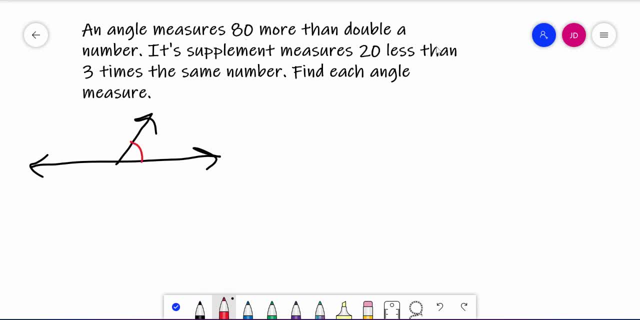 alright. so this one is 80 more than double a number, 80 more than double the number. so be careful: 2 x plus 80, it is this one, this one, this angle right here is 20 less than three times the same number, so 20 less. 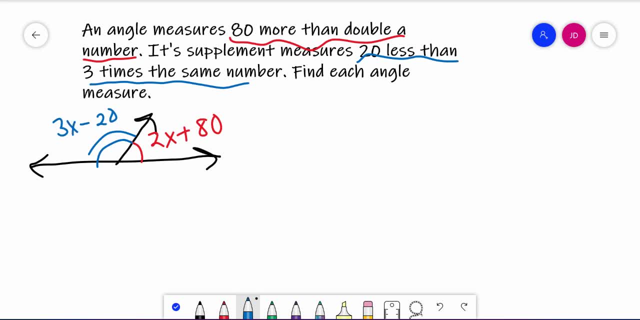 than three times the same number. all right, we make our equation: 3x minus 20 plus 2x plus 80 is 180. combined like terms, 3x- 2x is 5x negative. 20 plus 80 is 60 equals 180. 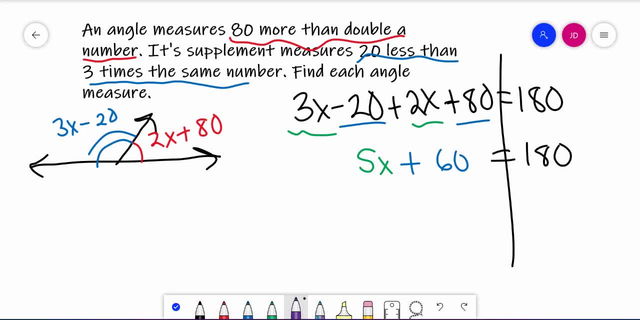 minus 60 from both sides, and we get 5x is 120. divide both sides by 5 and you get x is 24. all right, now we have to plug it back in. i'm going to use the calculator three times: two times 24 minus 20..